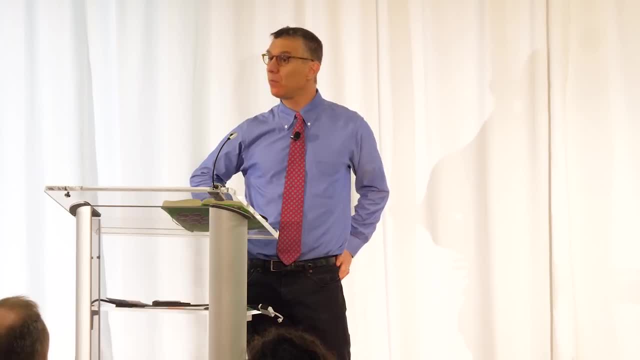 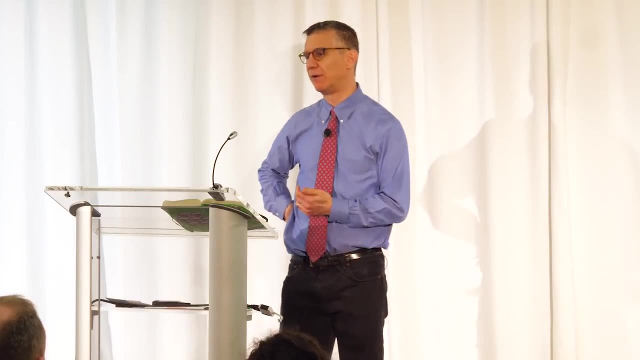 of three teaching assistants for Fred Mosteller, who had been teaching introductory statistics at Harvard for 30 years, had written many books. He took us to lunch every week And I remember once he asked us our opinion on some. I can't remember some education thing. 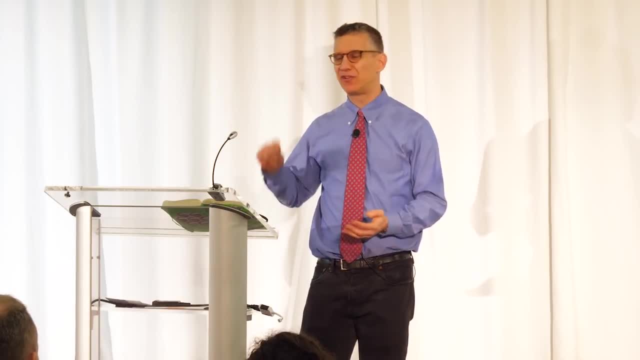 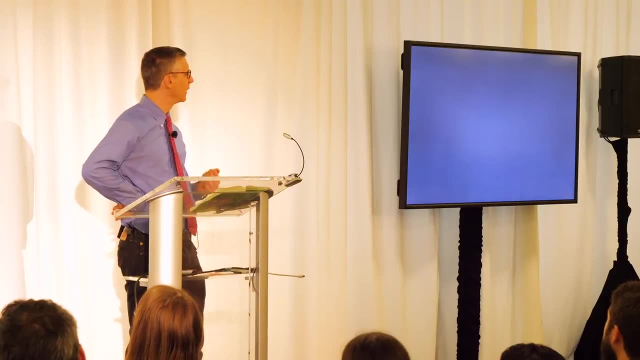 like what should be done, blah, blah, blah. We each gave our opinions and then he just snapped right back at us. He said: that's not what you should do. I said: what do you mean? And he said: when somebody asks you what you think, it's not because they care. 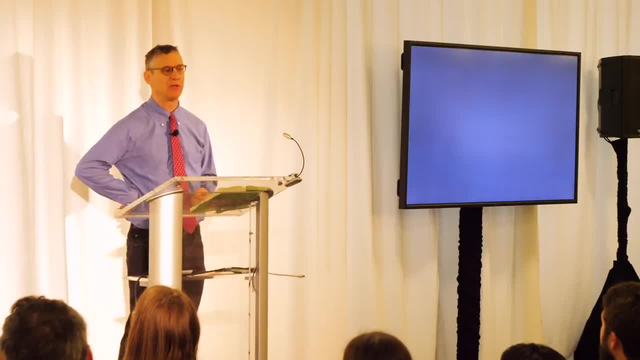 what your opinion is. They're asking you as a statistician, So you should answer by suggesting how you would design a survey or an experiment to study it. That's why they're asking you. Or maybe we could say more things like: maybe you could design a measurement error model. 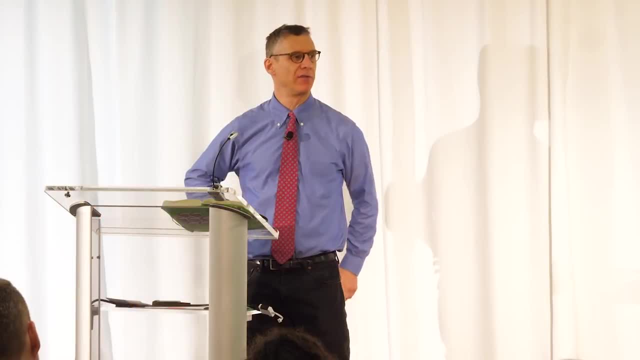 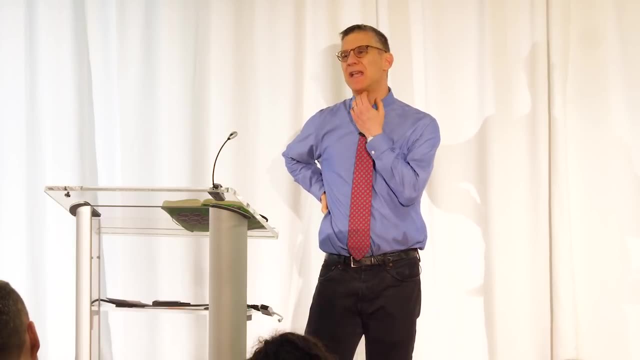 or whatever, but the same principle. Now, the other thing he told us was that you never know what people are going to get out of your class. So he said he would teach different things in different years and sometimes he would run into a student years later and it turns out they didn't get anything out. 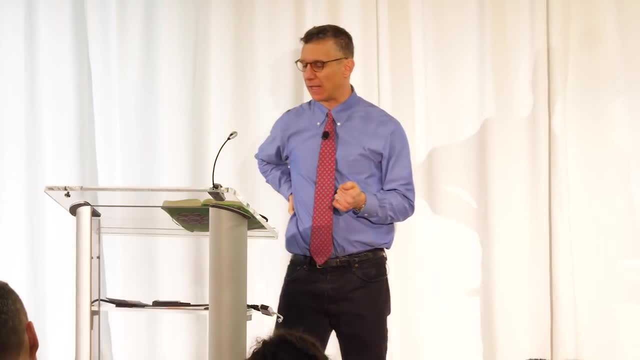 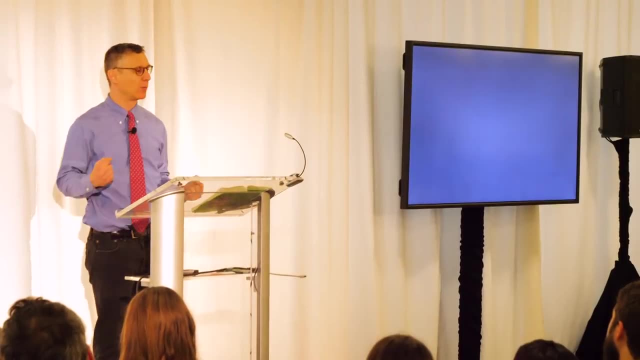 of his class except one throwaway remark, and it changed their life. So you don't know what it's going to be. So when I teach, I always say I need a take-home message in every class, Every class. what are we going to do today? This is what we're doing today, and 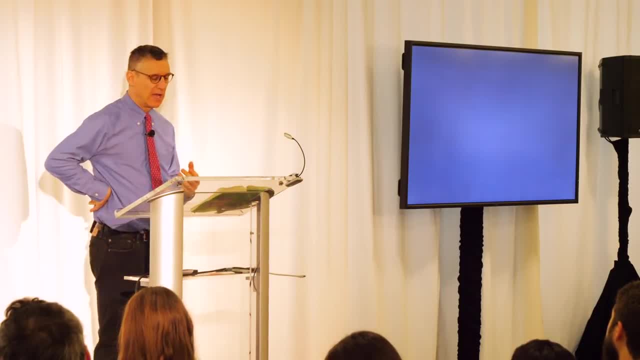 you're going to get something out of it and come home right away With this message, And so I thought I have to do that for you. You came, you paid Jared your hard-earned money to hear this. You're not here just to be entertained, You want. 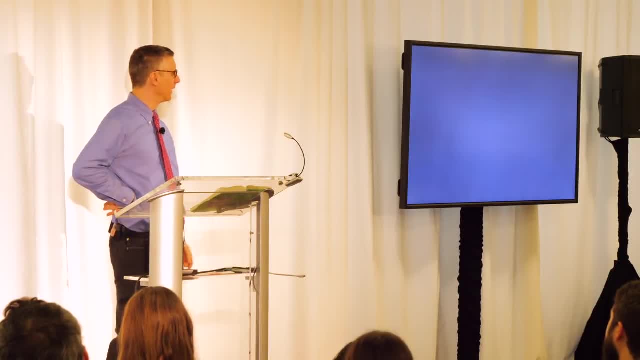 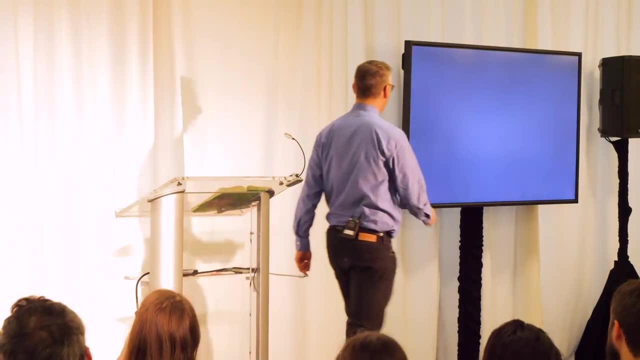 to learn something useful. So what could it be? Well, like R tips, Maybe not. You all know more about R than I do. There's a graph here. I guess I can draw it here. So the x-axis is what's the x-axis? 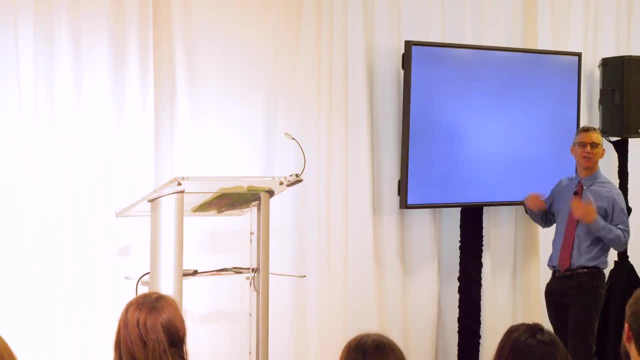 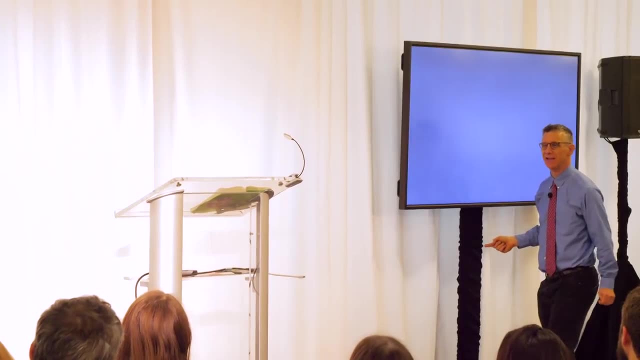 What's the x-axis? What's the x-axis? always Time, Time, right, right. The x-axis is time. The y-axis is like how good you are, And then it's like how good you are at R, And here I am gradually improved. Well, I started. 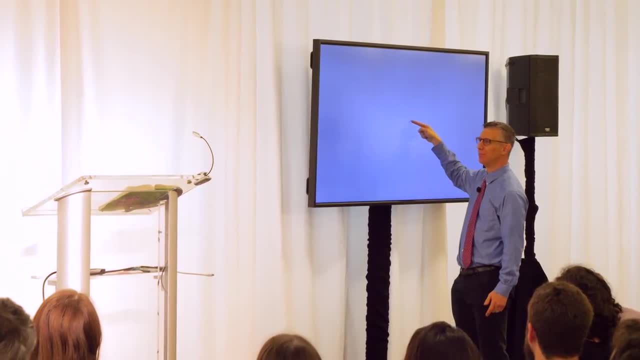 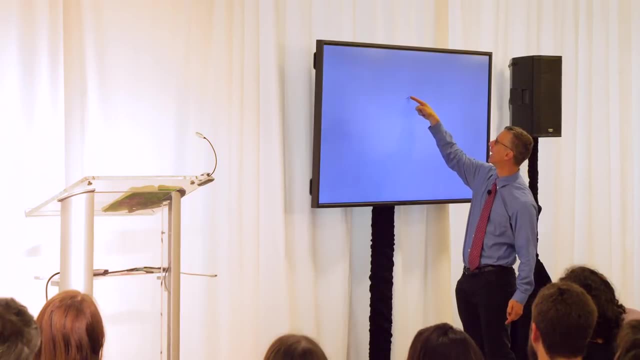 using S, but same idea. So I gradually improved. Now here you are. I've been improving right. Here you are, who started 20 or 30 years after me and you're up here right. So for me to 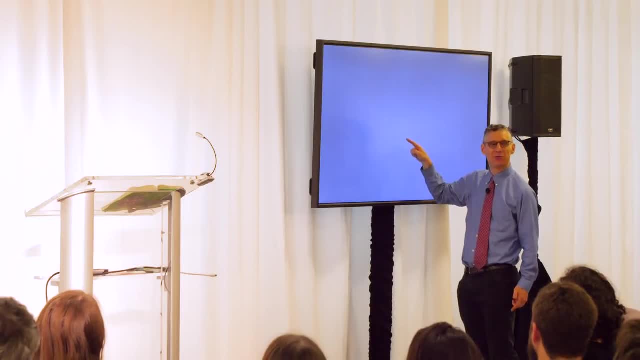 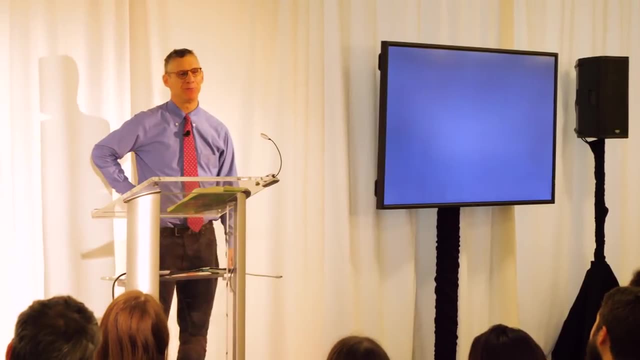 say, hey, look what I learned just now. This is stuff like: hey, I learned a new trick in base graphics. You want to hear it? I mean, what next do you want? What do you want like Space Invaders, cheat codes? 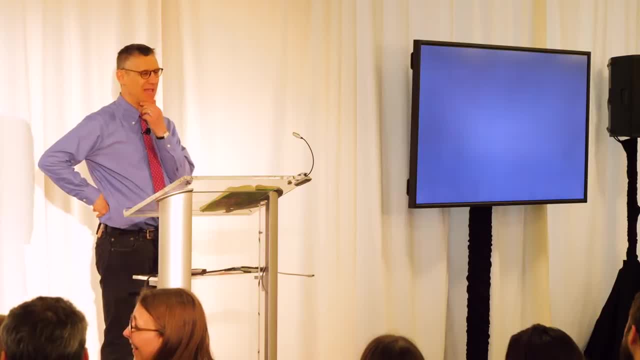 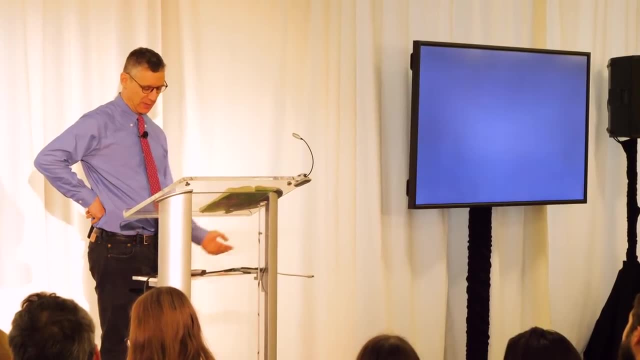 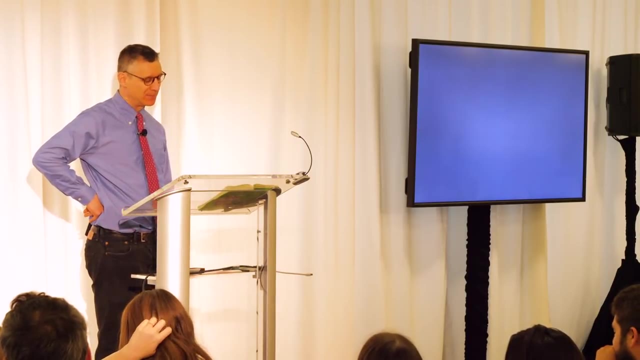 It's not going to happen, So I can't do that. Well, I could tell you about Stan, but I think maybe that's too wonderful to waste on you right now. Maybe next year, Jared, if you invite me back. So here it is. I'll tell you something that you can take home. You can. 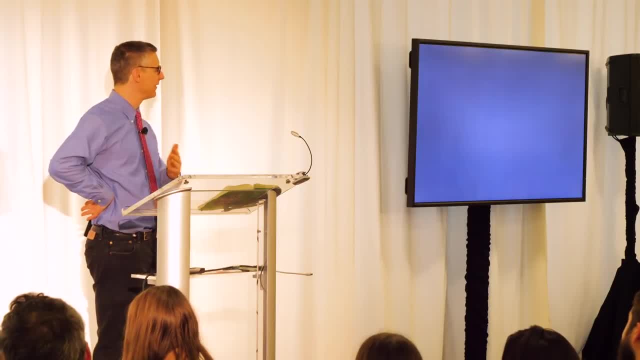 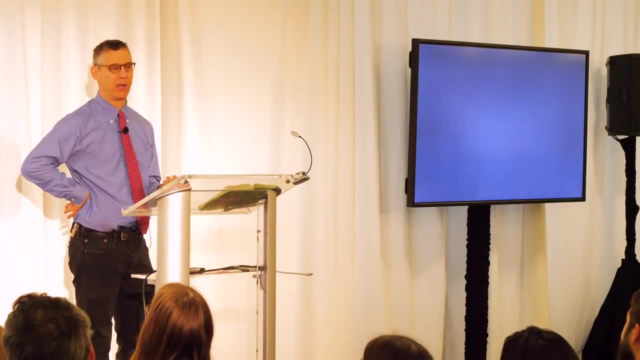 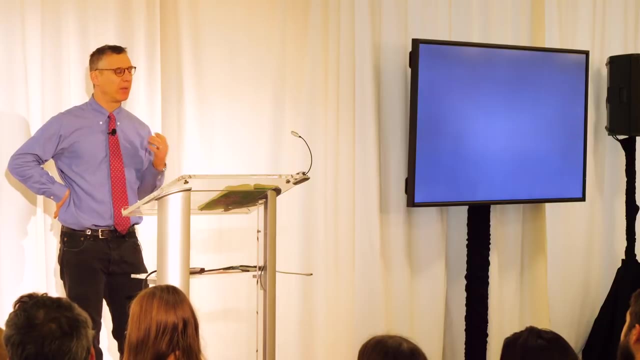 take to the bank and succeed with it. It's this thing you might not have heard of. It's called p-values And what you do is you run an experiment. Now it's kind of important that you do an actual randomized experiment or a random sample survey, something with probability in it. 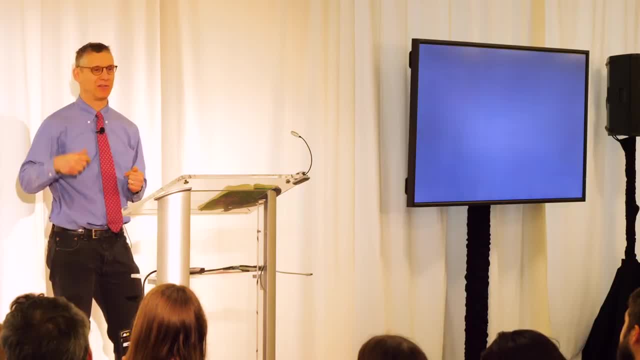 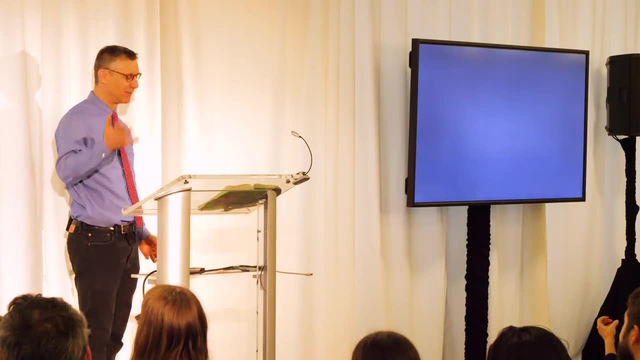 because there's a well-known principle in applied statistics that a chain is its strongest link, Right, You see? yeah, exactly, You have to think that one through, Then you laugh, right Tenth, it's not really true that the train 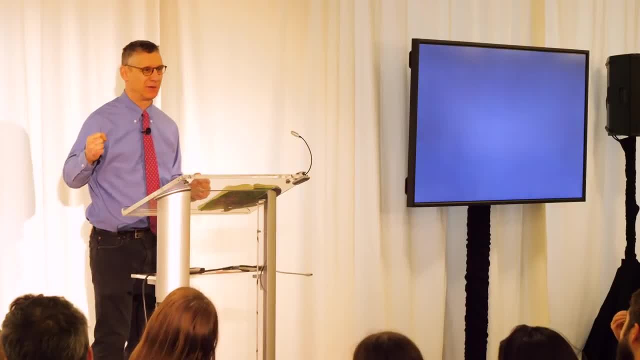 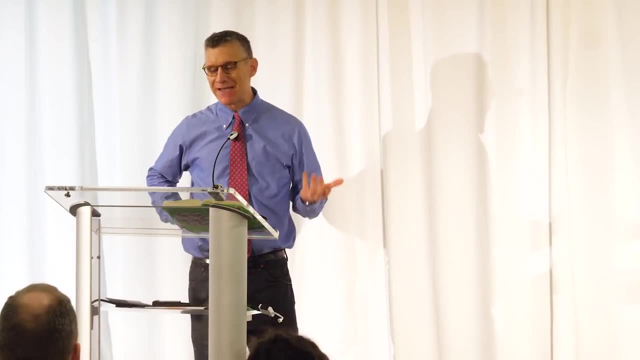 But this is how people act. So the idea is: you need that, You need that identification, That's your key to the kingdom, And then, once you're inside the castle, you can ransack the place right. So run an experiment, okay, Then you have a pile of results. So for every. 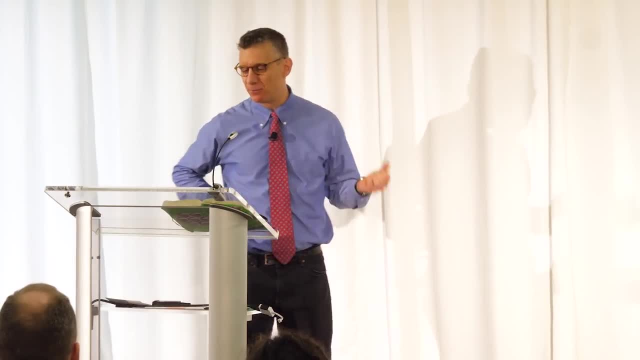 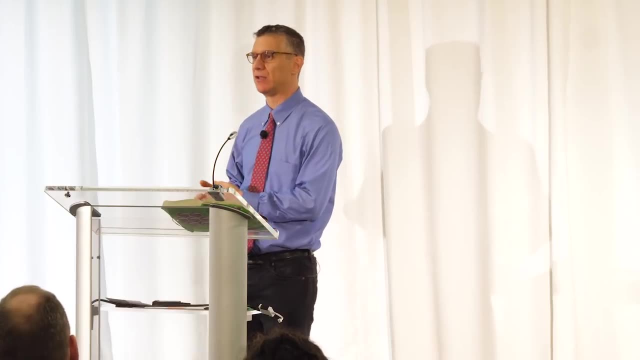 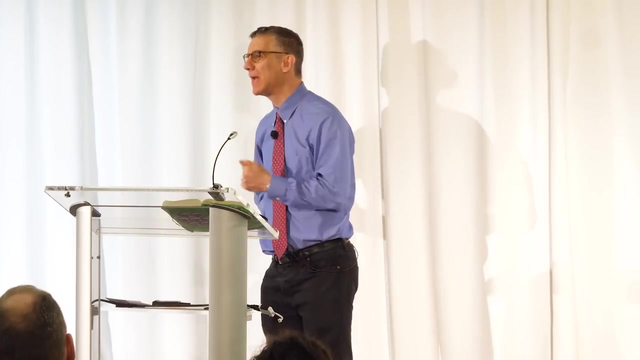 result: you have calculate a p-value. If it's less than 0.05, you've found something real, You've made a discovery, all right. And if it's more than 0.05, then you've proved that something is zero. and so either way there's a win. but you can get a little. 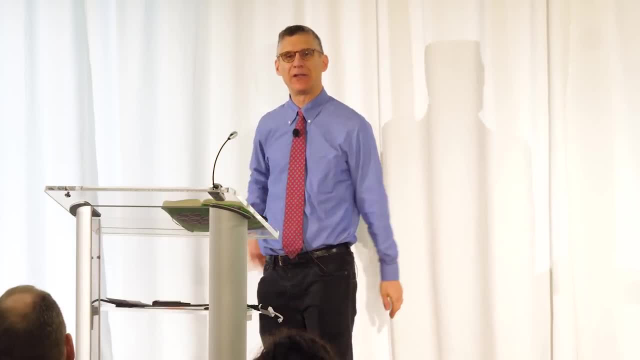 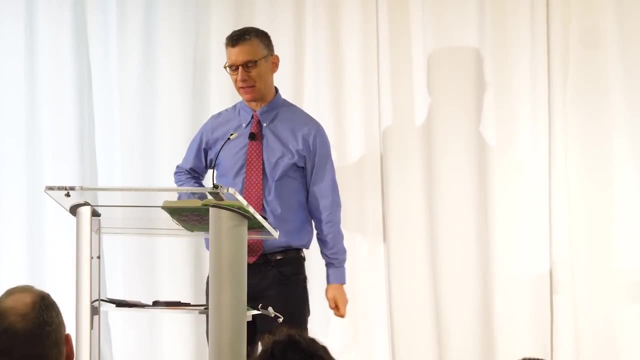 bit more out of this. I there's another little trick you can do, which is, if it's if the p-value is, or like, between 0.05 and 0.1, you can say that you've discovered that it's a small effect, and then you can get entire patterns out of. 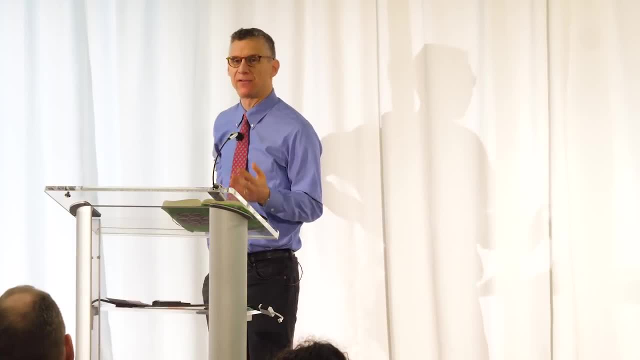 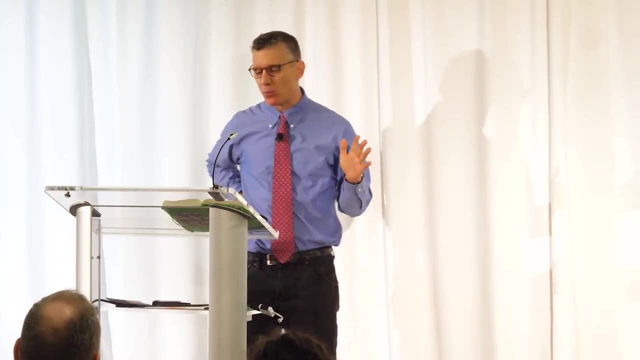 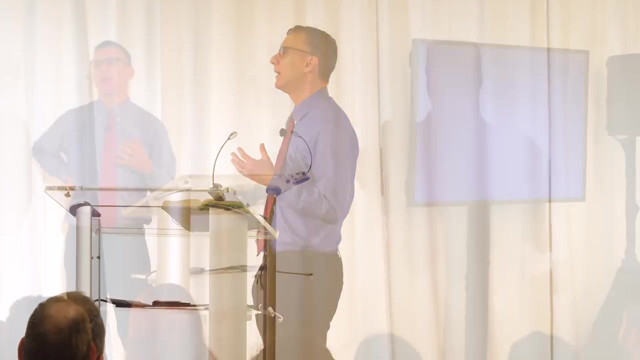 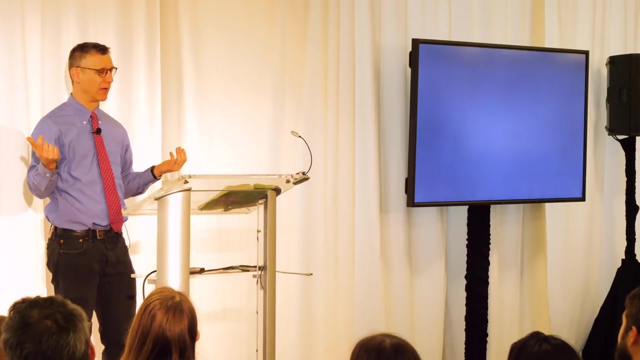 this now you might worry if you do that, this, you might worry that your, your measurements might be too noisy, that these, these things might not replicate. but don't worry, okay, don't worry, because what do we care about? we care about two things in life: right two, only two things. 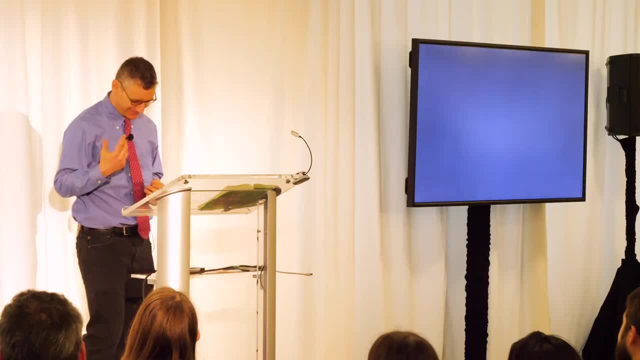 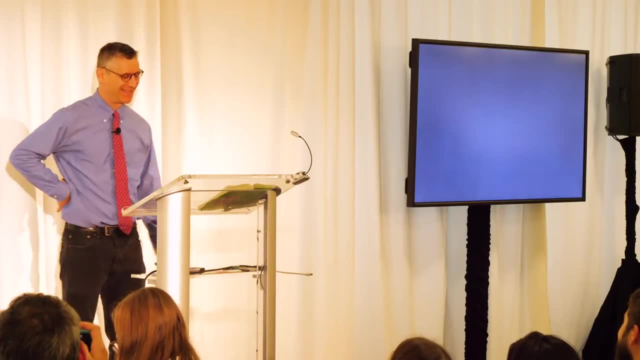 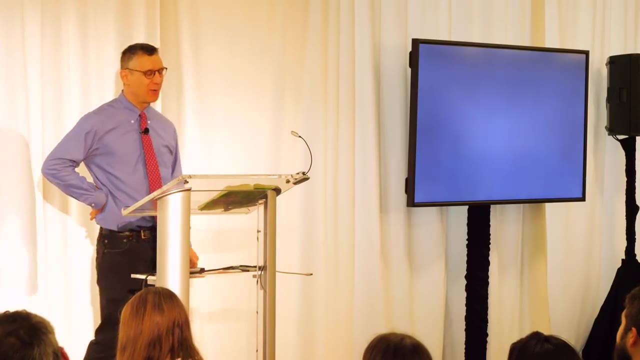 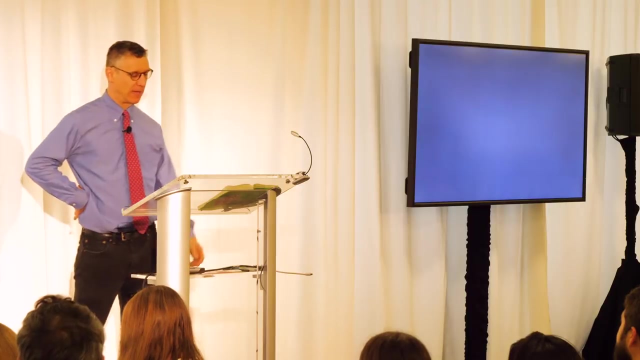 in life for reals. bias and variance right, but I mean that, I mean that like I mean. I don't necessarily mean it the way people always mean it, but I mean it. now you don't have any bias because you remember you did a randomized experiment, so therefore you have no bias. you also. 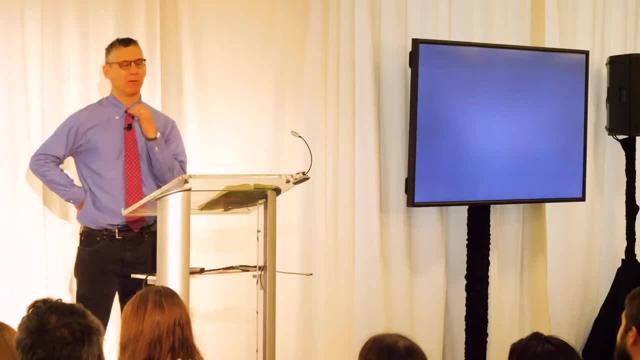 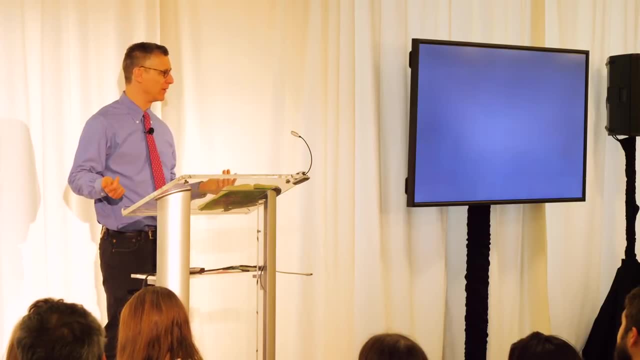 have variance. well you're. the problem with variance is if it's too big. but why is it a problem of variance is too big? because that means your power will be too low. why is it a problem that your power is too low, that you won't get statistically statistical significance? luckily you've. 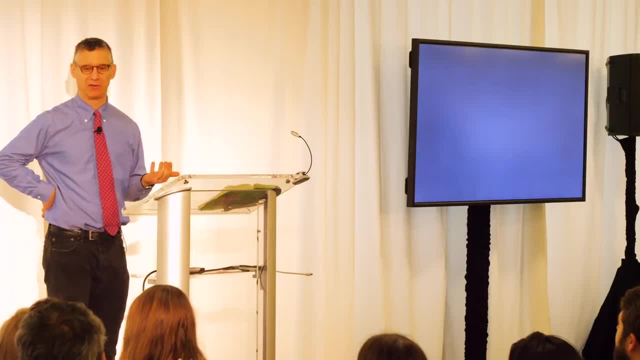 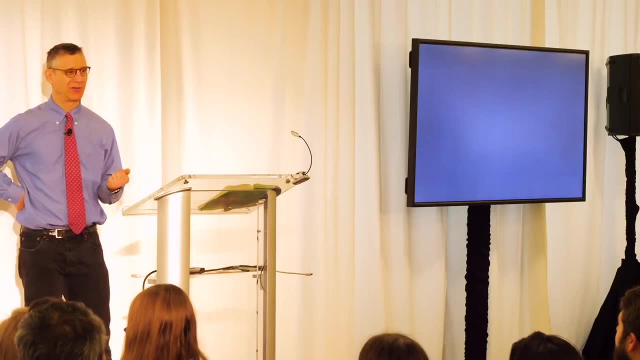 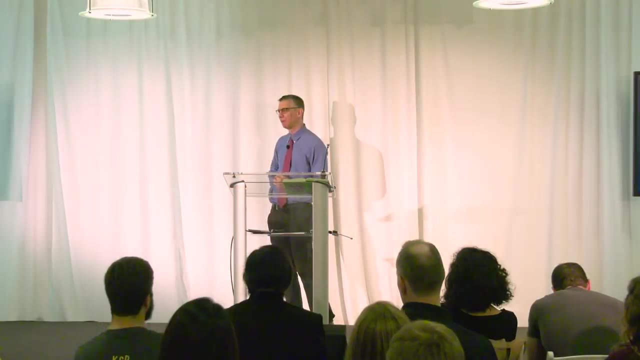 you followed my advice and you've looked at enough things that you've found statistical significance. therefore, retroactively, your power was just fine. right, this is you know. this is this is what we're gonna say like in a couple weeks. right, you know the Warriors didn't need Kevin Durant. you know they. 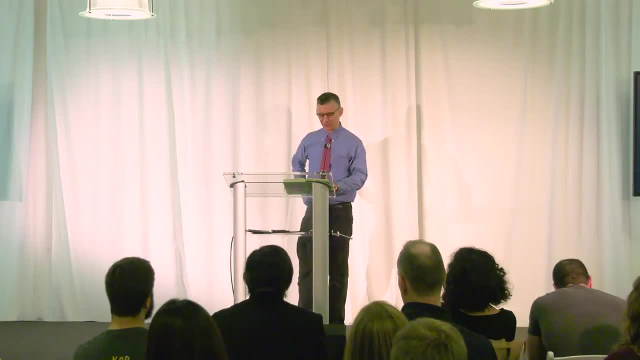 know, whatever it is right, okay, the the power is is just fine. so therefore, your measurements were good enough, So you don't have to worry about that. Now you maybe think I'm speaking ironically and you might say this might work in academia, because the goal of academia is to publish a paper. Okay, so it's a. 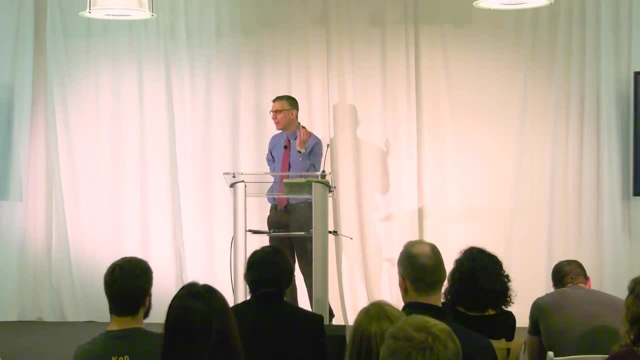 little like academia is like sports. right, you want to win the game. once you get the W and the one more in the W column, the game is over. It doesn't matter if you deflated the football. whatever, it is right. I'm sorry about that. just that Jared told me I had to mix in sports analogies because he was 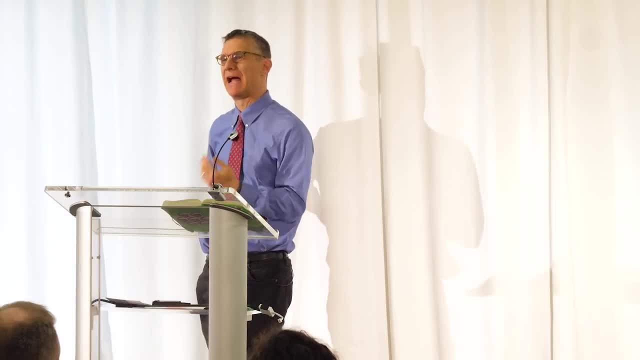 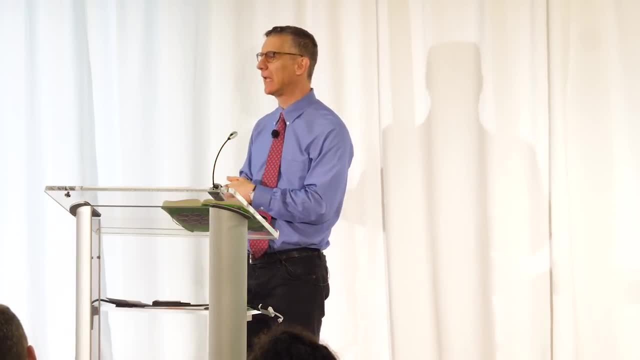 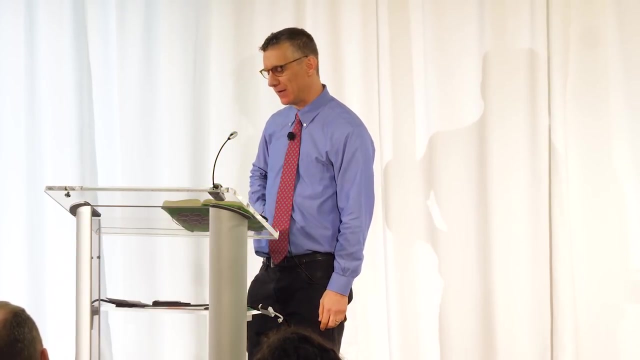 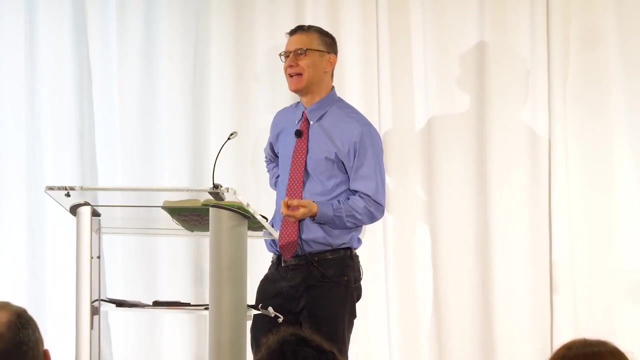 Talk about sports and how it's an approach that he sort of you know they get to speak for it. once you win the game, it's over in real life. You all mostly work in the real world, whatever that means, And there it's more like a game of ping pong. 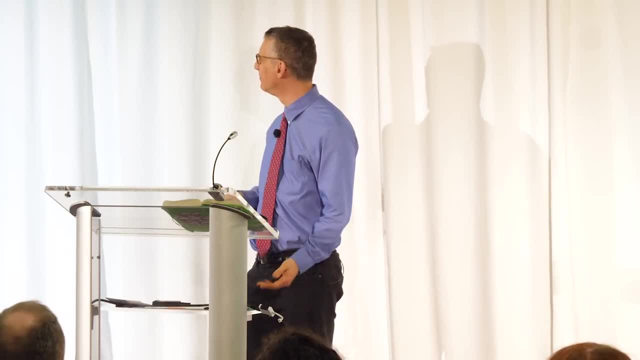 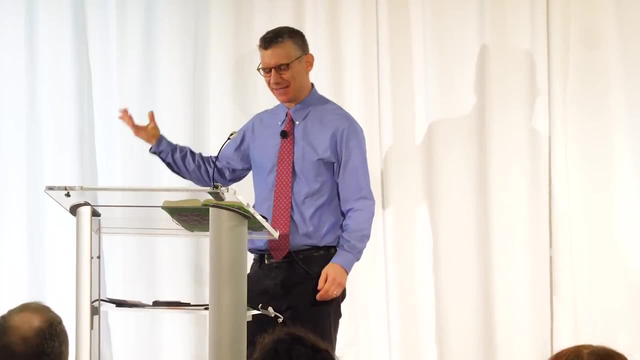 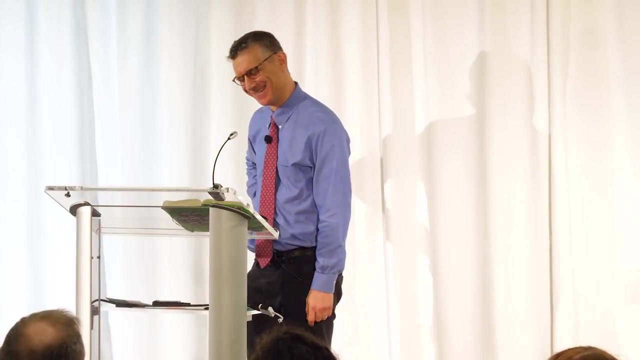 You want to keep scoring points And I don't know Ping pong, John, I don't know. It looked better in the slides. He wouldn't let me use slides either. That was another thing. So it's a little different, because your goal in business, 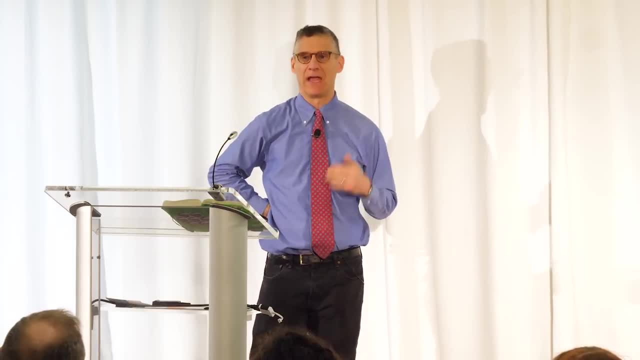 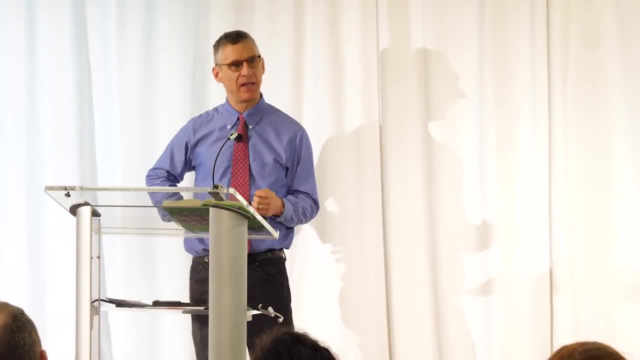 is to make money. Maybe you're not all in business. Your goal in government is to help people out. Often it's to help people use the services available to them In nonprofits. you might be working in medicine. You really want to change things for the better. 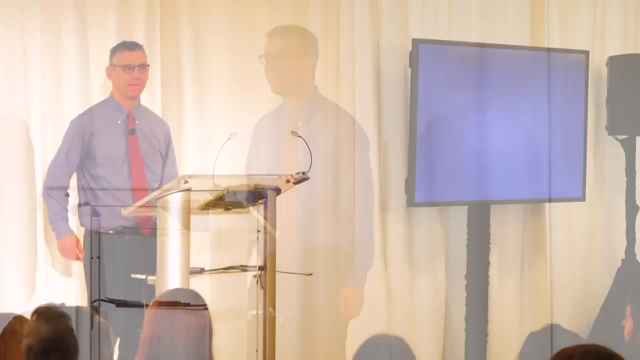 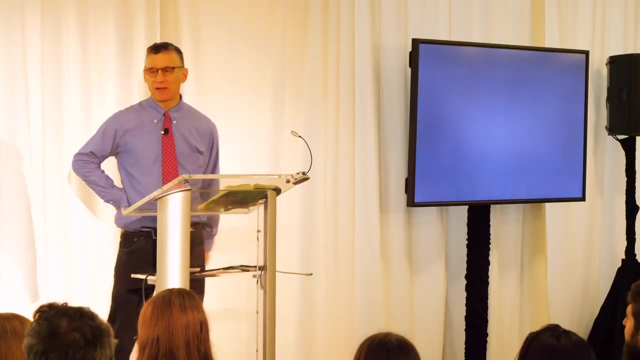 It's not just ratcheting up wins, It's not just about having a fancy CV. It's about things that are going to count. It's about things that are going to count to somebody, to real stakeholders. But actually, this trick I told you. 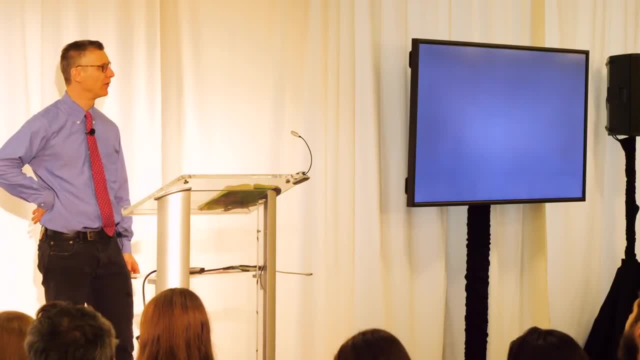 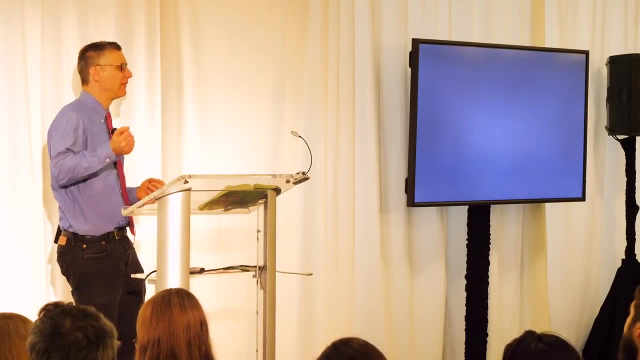 about the statistical significance. it kind of still works in the real world And I've seen that. I've talked to people They're doing A B testing And they're like, yeah, we set the threshold down to 0.8. 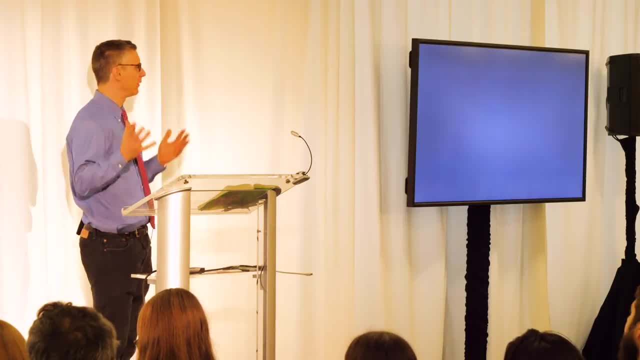 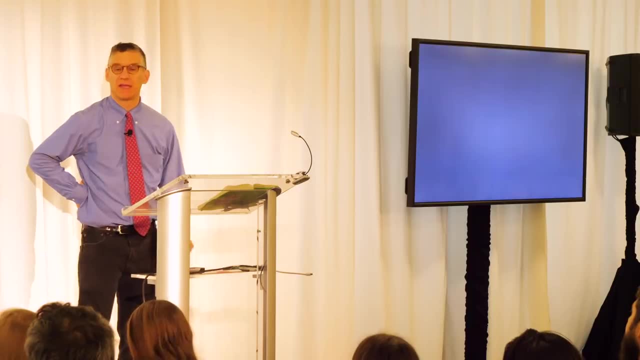 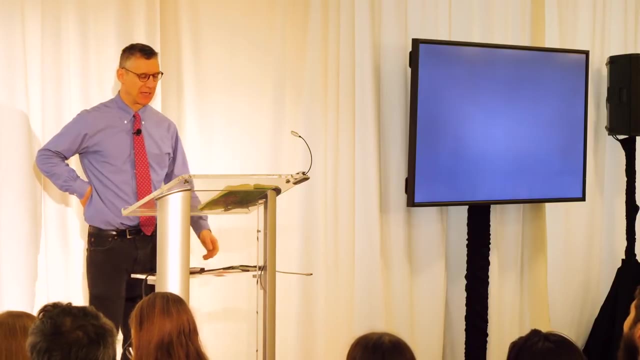 instead of 0.95, because we wanted to get this. You can use these tools to succeed. It's kind of cool because it's like alchemy. You've like: Yeah, We've converted randomness into certainty. But there is a principle. 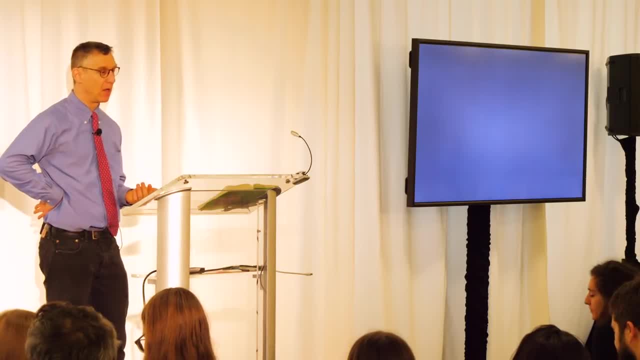 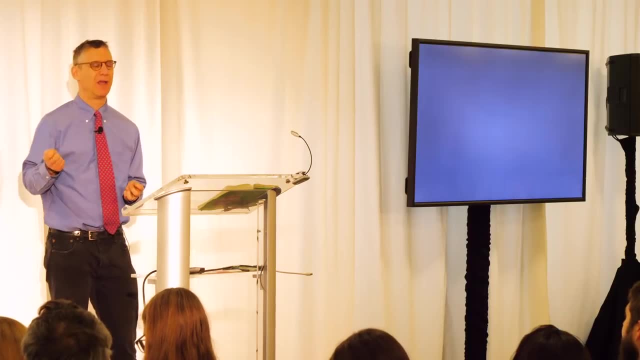 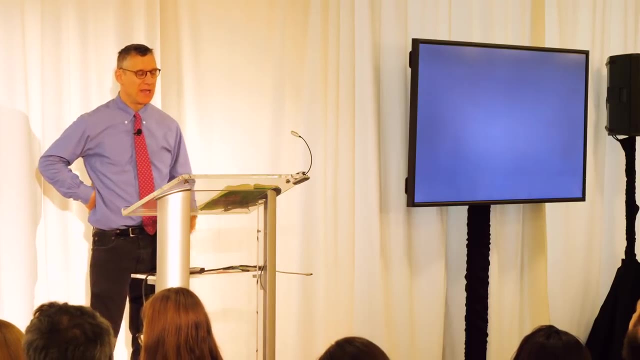 We sometimes call it the conservation of variance, which is that the variance has to appear somewhere else, Right? So the flip side of taking something uncertain and pretending it's certain is that it will fail to replicate later. Right, The variance has to go somewhere. 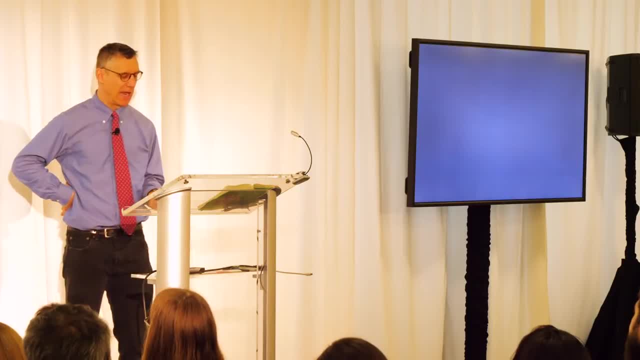 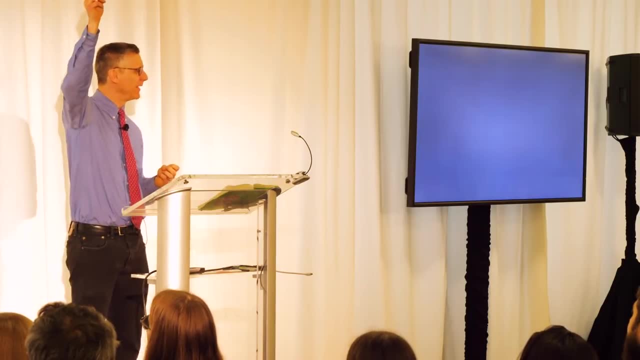 And that's why you could say: a lot of statistics is like a pyramid scheme and you really want to get in on the ground floor, which I've never really understood. that because in a pyramid you want to be on the top, because the ground floor is. 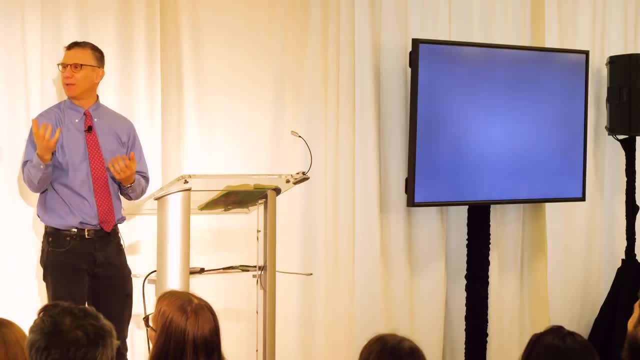 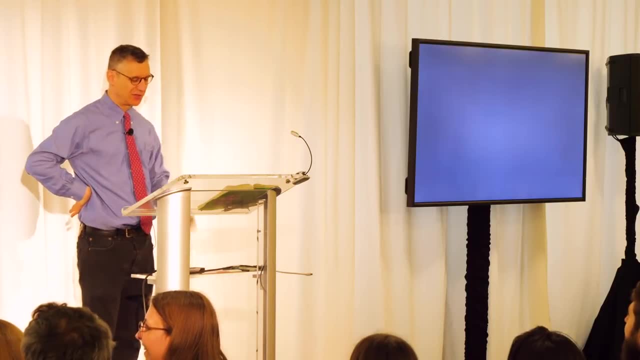 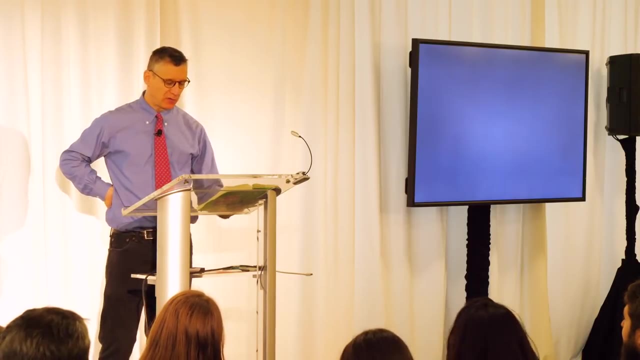 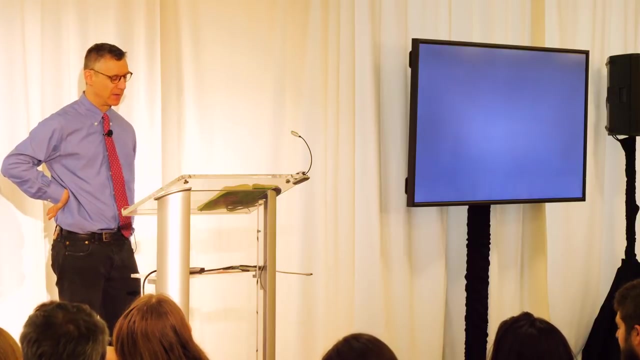 where all the suckers are, But they build the pyramid starting from the bottom. So I don't really understand the pyramid scheme principle. It seems to be just a terrible analogy. OK, So how can we understand this? There is a tool that we can use. 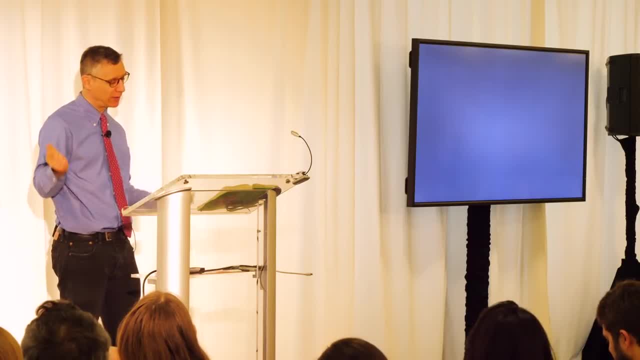 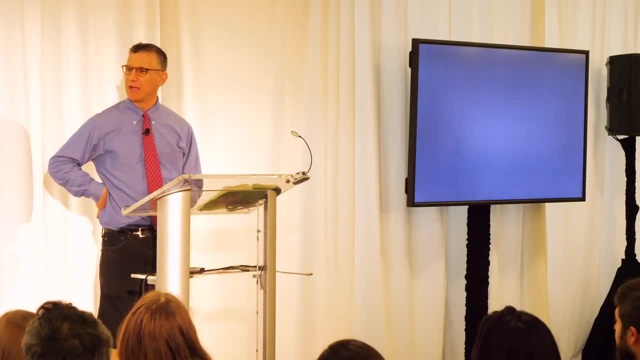 There's a set of tools like you could use, Python, whatever, But I'll say R because it's the R conference. I spoke at the PyConference, the Python conference, like a year or two ago, And I told them I didn't have any Python. 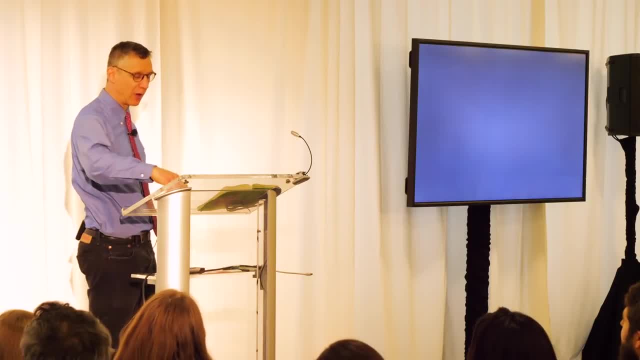 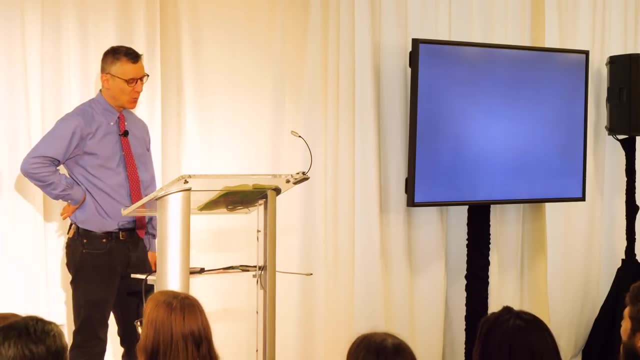 So like, is that OK? And they're like sure, It's just called the Python conference, It's not really So. I think this is probably similar. So how do we understand this? What we have to do is we have to simulate the world. 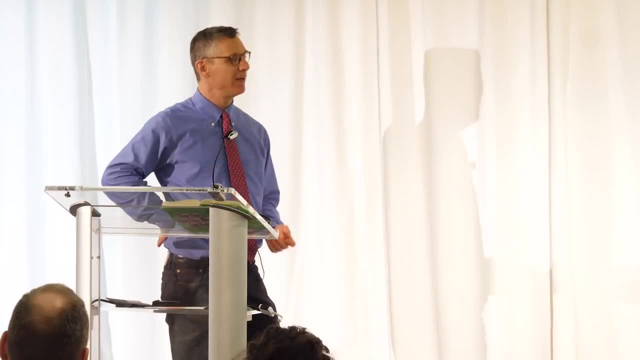 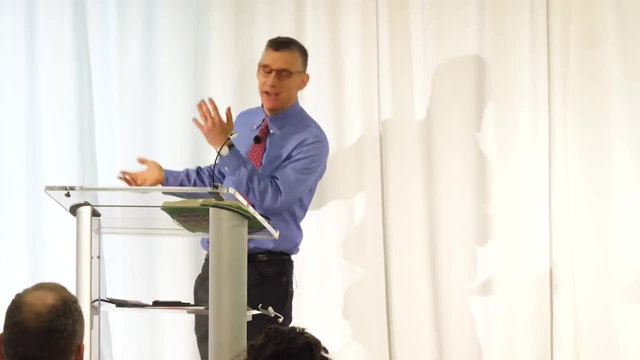 And I'm serious about this. So if I want to- I mean, this is kind of old school, Like you'd say- oh yeah, some thick-headed person doesn't understand the Monty Hall problem, so let's do a simulation- 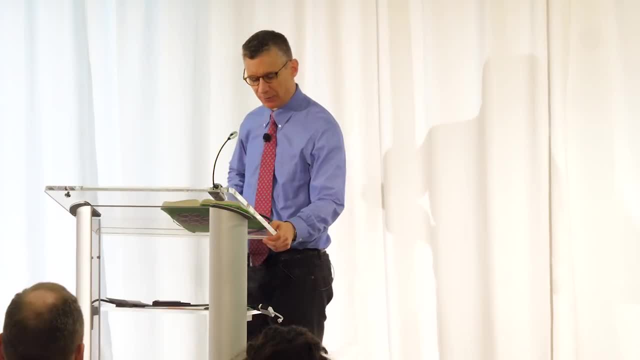 Like who cares about the Monty Hall? I don't like the Monty Hall problem actually, because I feel like it sends the message that probability is so tricky by giving you the answer. I mean, it's not really that tricky. 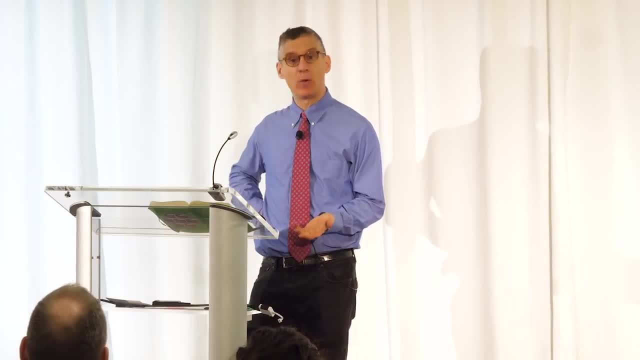 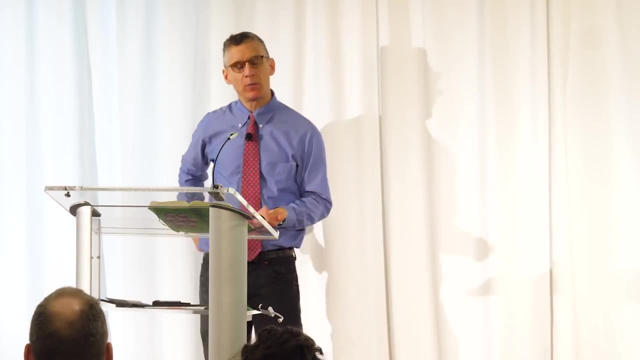 You can kind of brute force things. But if you want to understand something like what happens, if you call things statistically significant and then act as they're true and then do replications, what you want to do is simulate a world in which people behave in a certain way and then see what happens. 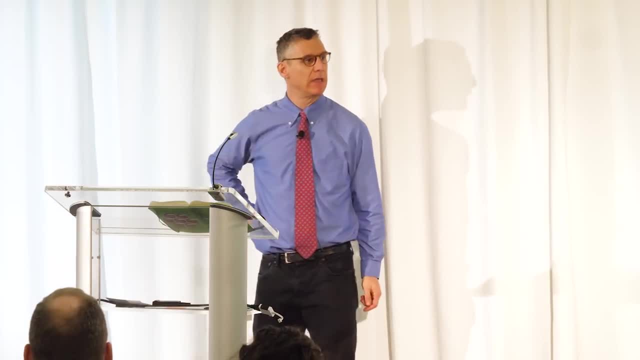 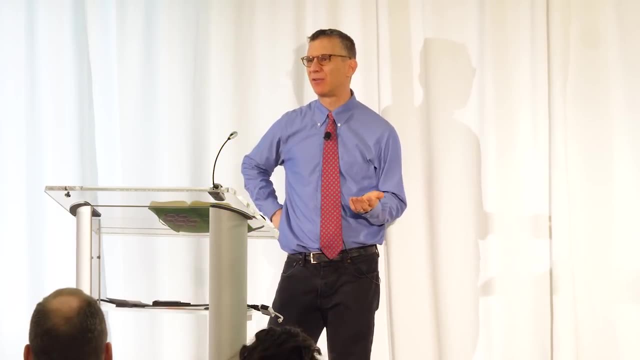 And you can see what happens. So if you're working in your company doing A-B testing and you want to use an 80% threshold or whatever, the answer is not 80%. Like to say that the answer is 80%. I mean that would. 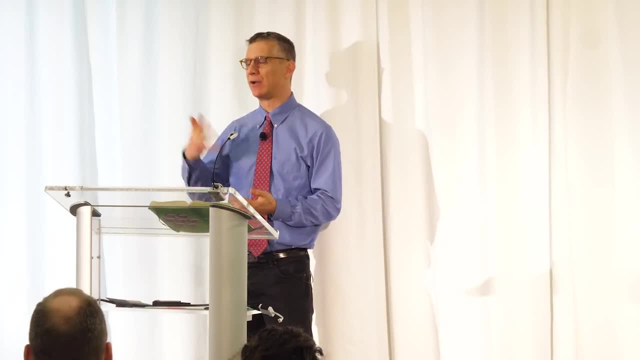 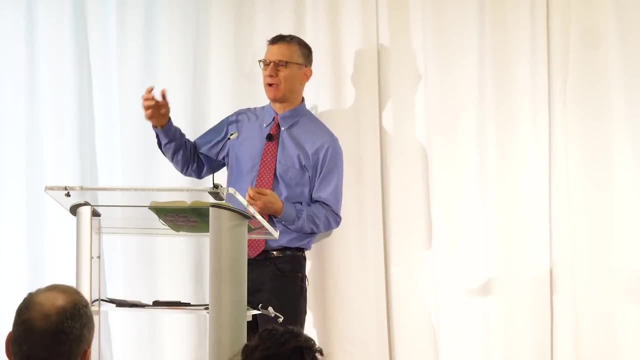 be like saying: like I'm a biologist and I want to grow a colony of like amoebas And I give them like a certain amount. I give them like two grams of amoeba food a day. 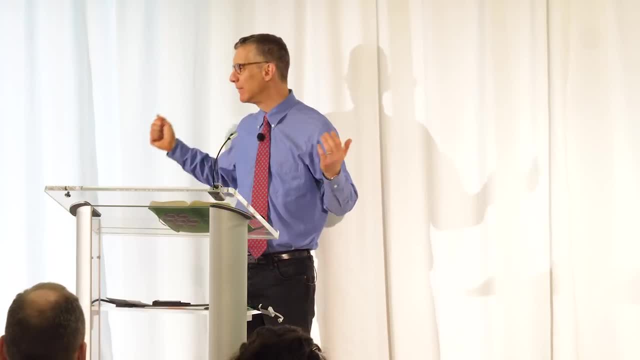 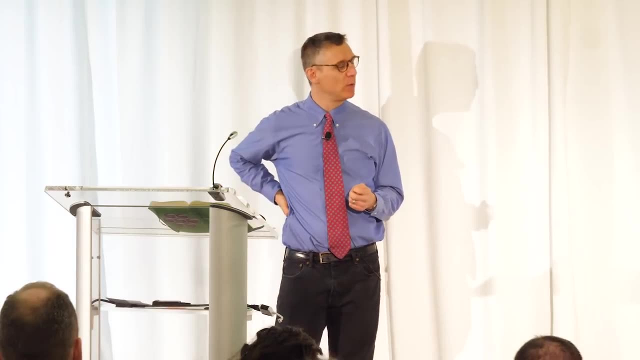 And like the answer to. like I said then, the question's like how many amoebas are there in three days? The answer is not: two grams of amoeba feed. That's the input, right. So, similarly, if you want to know, 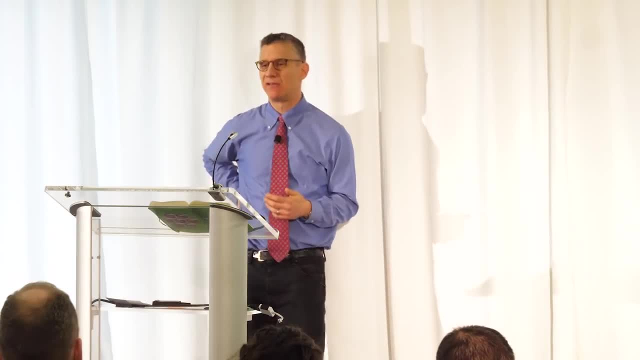 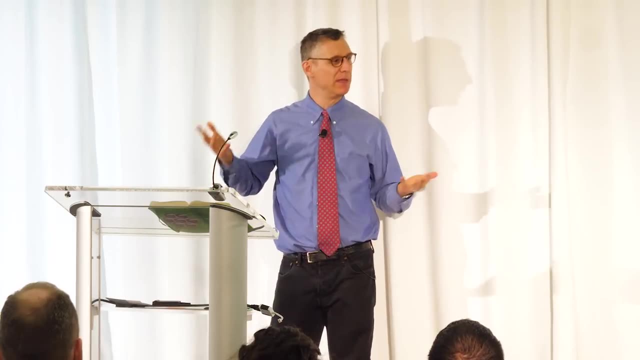 how reliable are your inferences? if you do significance testing with an 80% threshold, the answer is not 80%. 80% is the equivalent of two grams of amoeba food a day. That's the input right, The only way you're going to know the output. 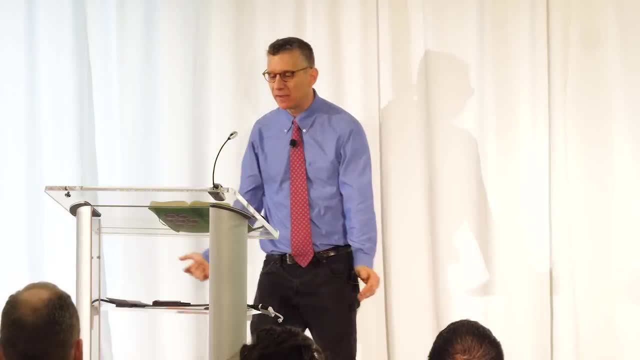 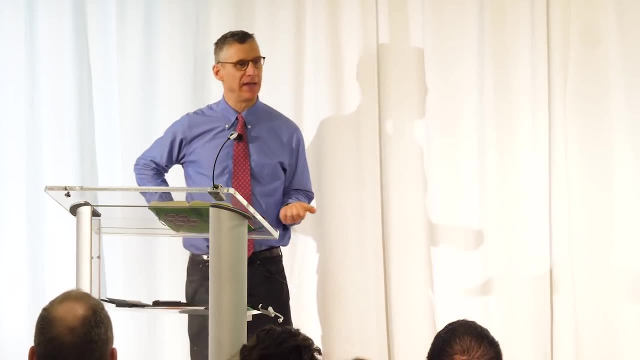 is to run the simulation, So you can do that. Now it turns out, running a simulation is hard, So it's a lot harder. it's a lot easier to analyze data than to simulate fake data, And even in statistics there's this funny thing. 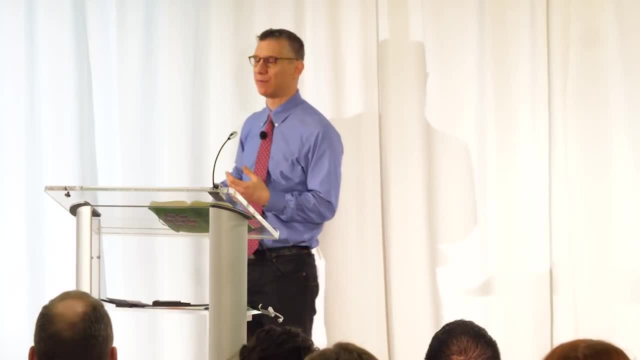 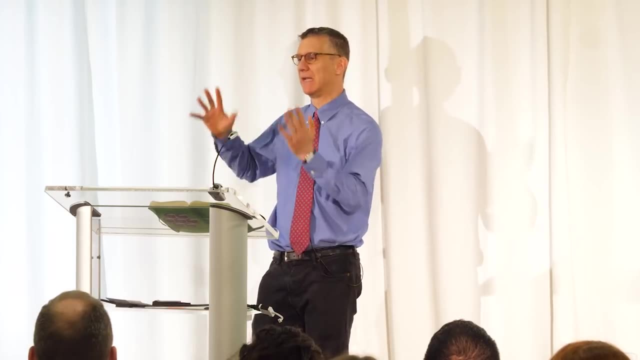 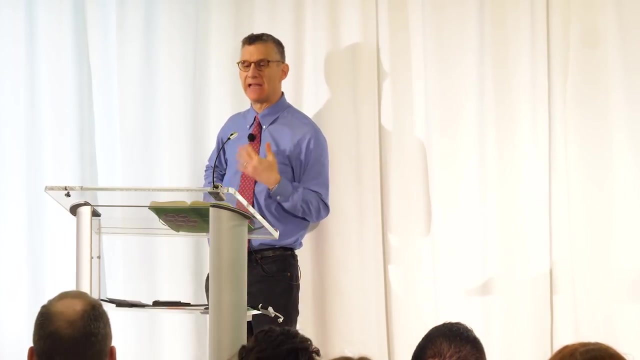 They talk about the likelihood. The likelihood is derivable from the data distribution, But the data distribution is more complicated than the likelihood. One likelihood could map to many data distributions, So it's actually it's easier to do Bayesian inference or just about anything else than to simulate fake data. 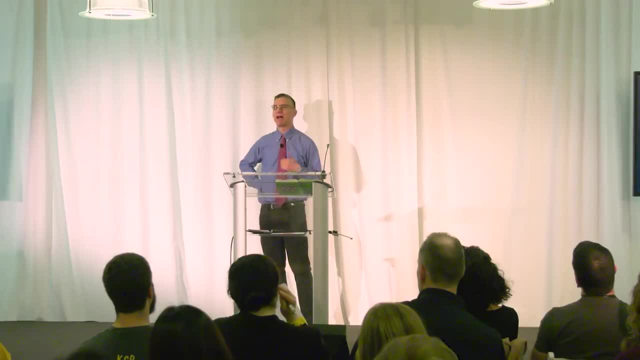 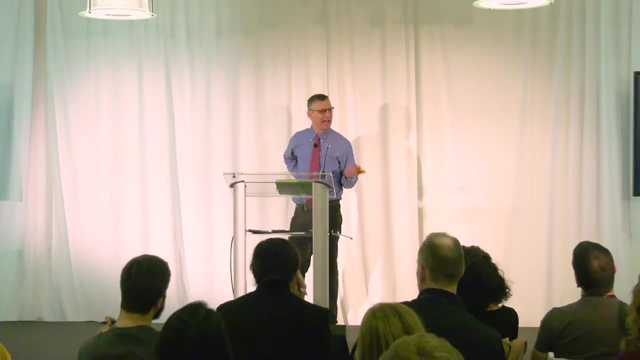 But only by simulating fake data. or obviously, sometimes you can do it through math, but that's rare, right? So only through simulating. You're like laughing- and that wasn't a joke- Like I got you all on the edge here. 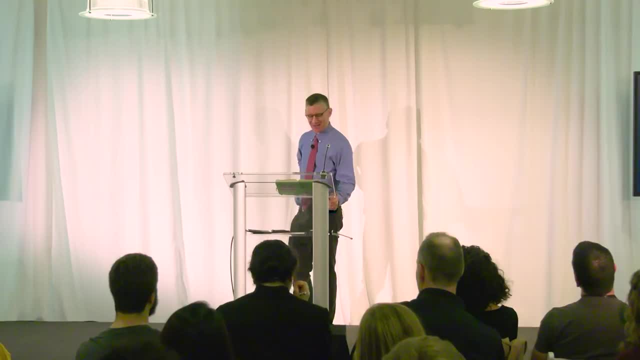 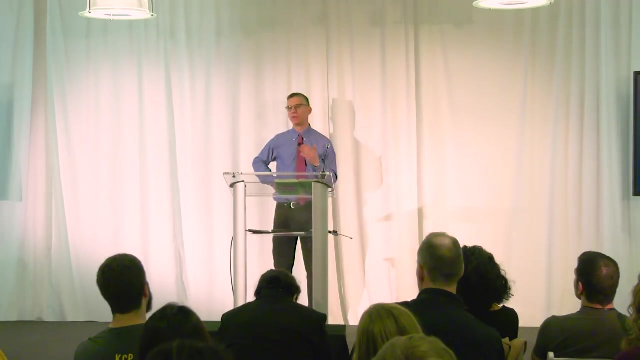 I could say anything at this point, So no. So to simulate the fake data, you have to simulate a system. What does that mean? if you're doing your A-B testing or whatever you're doing, You're working for the government and you're trying to improve people's use of social services. 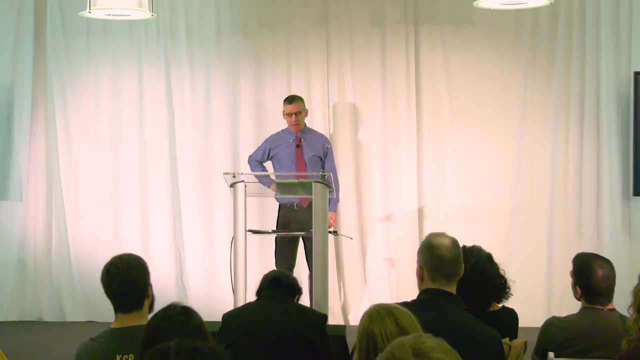 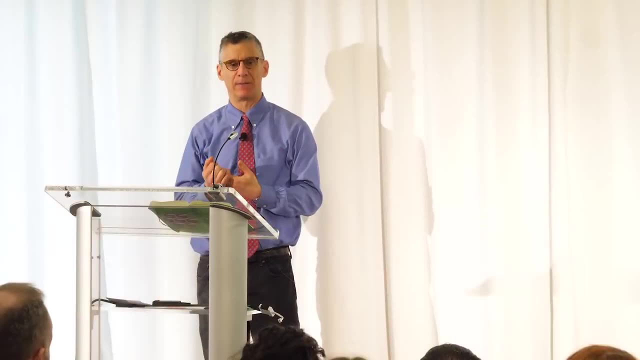 or whatever you're aiming for. You have to have a model for the world. You have to say: if I'm doing the A-B testing, well, how big is the effect that I'm testing Well, what's going to happen? 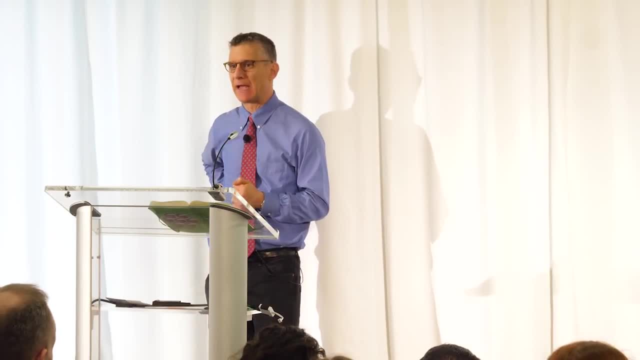 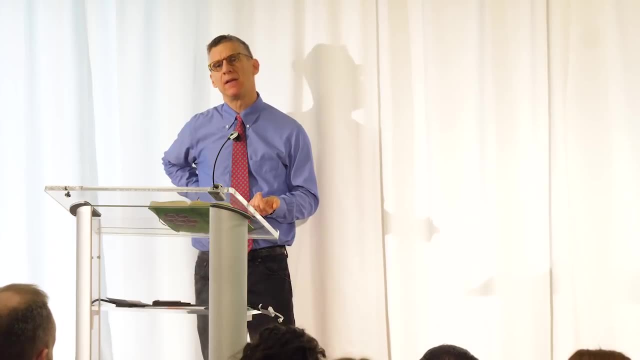 Statistics is said to be the science of defaults. OK, So the difference between, say, a statistician and I don't know like? there are physicists who work in probability And what they'll do is spend 10 years working on one problem, a really hard problem. 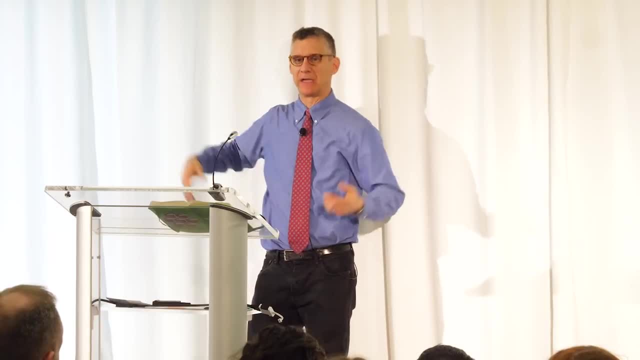 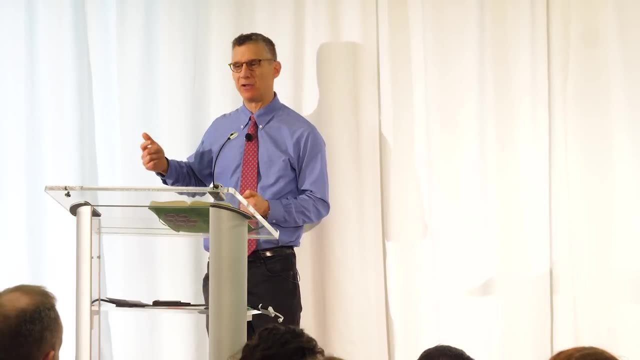 building a lot of scaffolding. I mean, they're building the Chrysler building, as it were, And that's a career. Statisticians, we're more like the guy who made Levittown like, except without the racial Exclusion and all that where we just 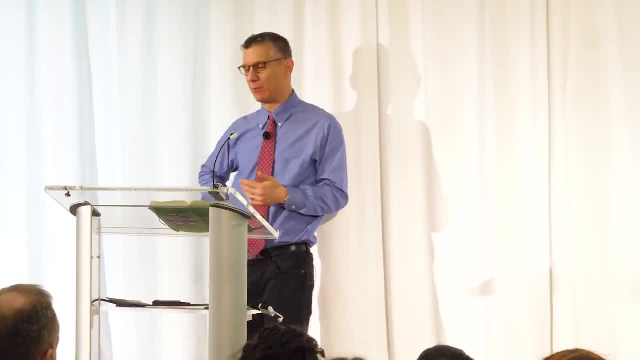 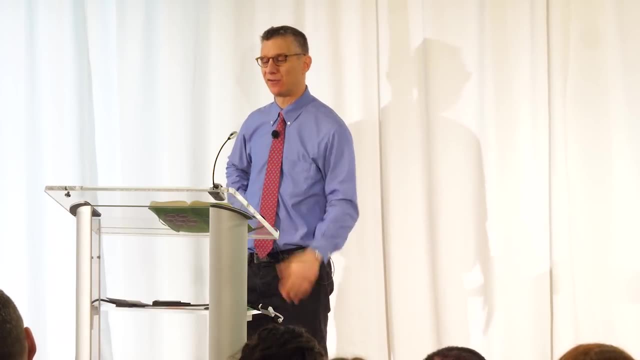 built. we want to build a lot of tract houses. That's kind of how we think. OK, So you have to imagine someone is going to do this procedure. What was it? Solve all your statistics problems using p-values. I think that was the. you know that Jared gave me that title. 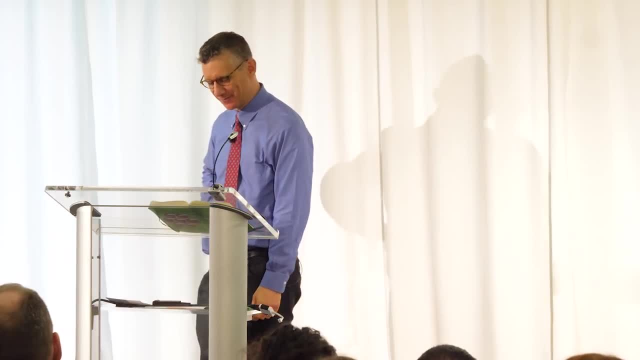 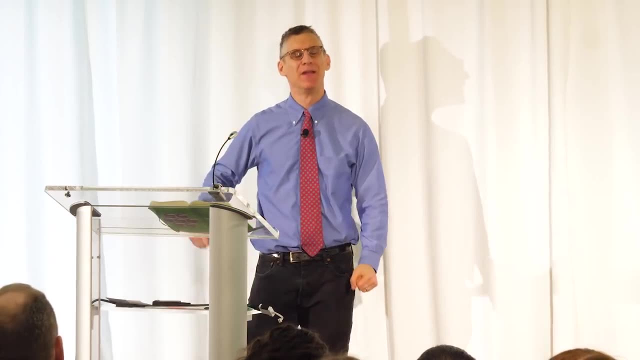 and said: go from there. So this is really all just up to his fault. So he's like: you can't get out of this one. Yes, I can, Jared, I tell you this time you can't trap me. 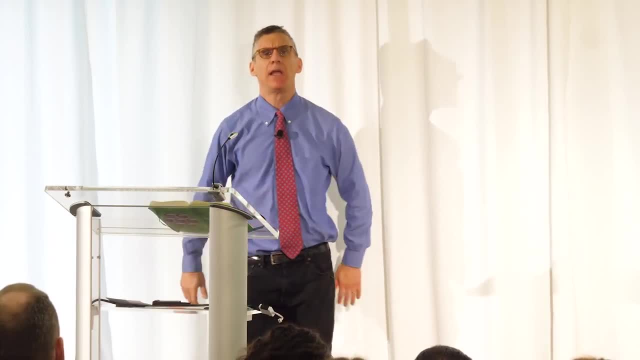 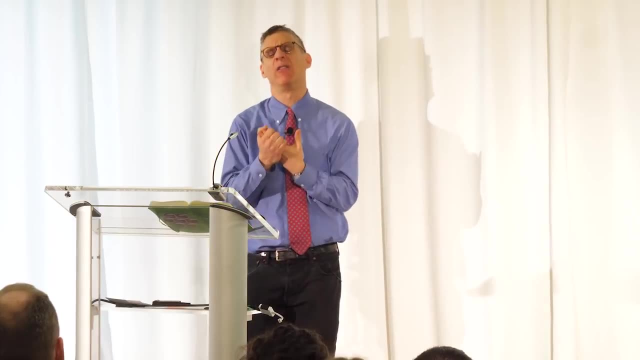 So it's not just OK. how big is this effect that I'm studying? You need to have a hypothesis about that And that's oh, this is really hard. What's my prior for the effect? I don't know. 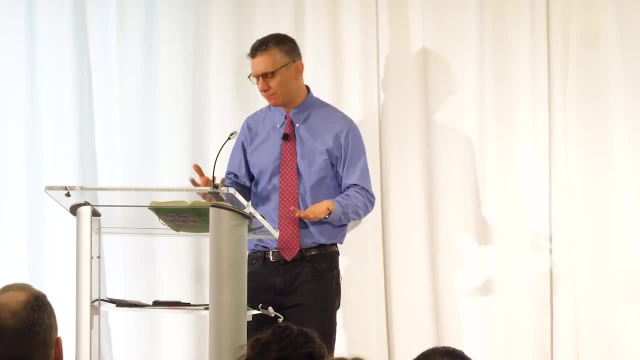 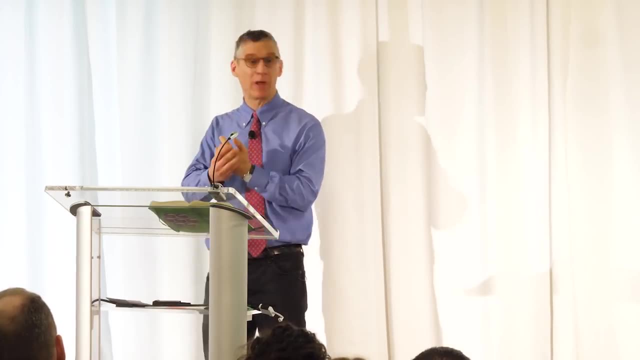 If I had a good prior for the effect, I wouldn't need to do the damn A-B test in the first place. You fool, You can't think of it that way. OK, The prior is real. OK, The prior is real. 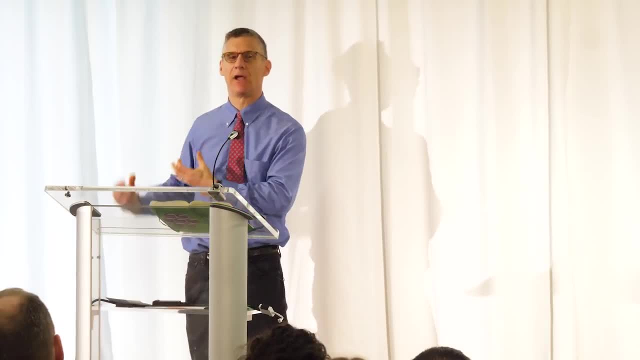 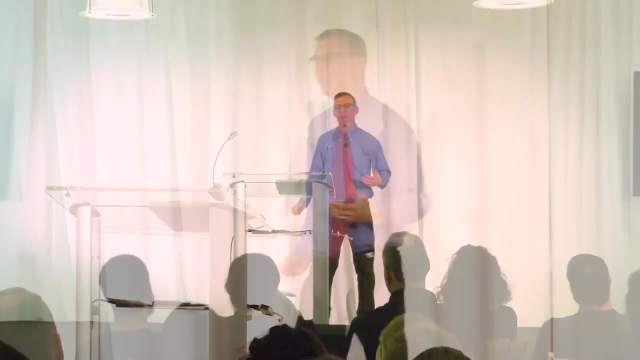 I'm like one of those holy rollers. you know, Like I feel, God, you know, whatever I feel, the prior It means something. It's the distribution, It's the distribution of actual effect. So you have to say like OK, all of statistics. 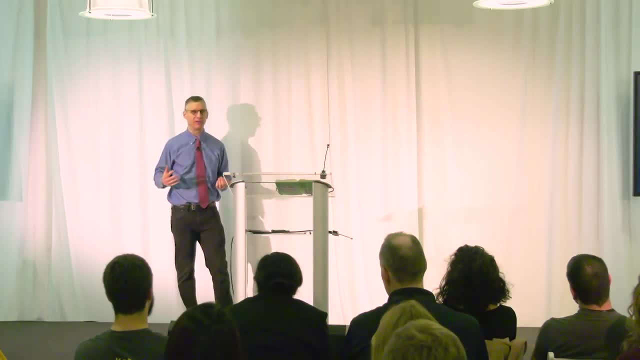 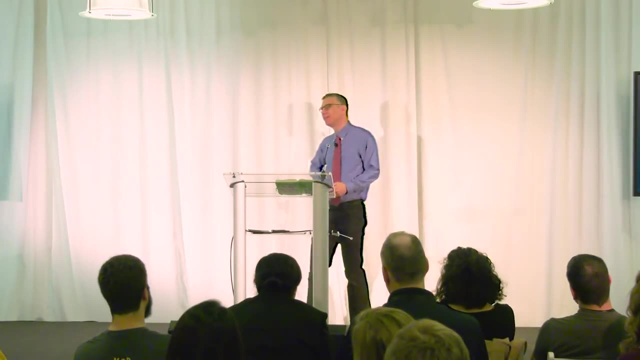 is about repetition, It's about the frequency- We're all frequentists here, OK. So the idea? no real, real. So the idea is there is a stream of problems you're working on. You didn't get hired to do one A-B test. 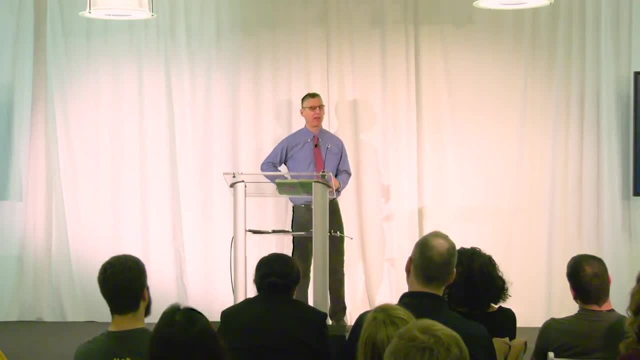 There's not one program you're rolling out. There's not one drug you're testing. There's a stream of these. Now, in a usual talk, I would start saying, OK, what's our prior for this? How do you validate this? 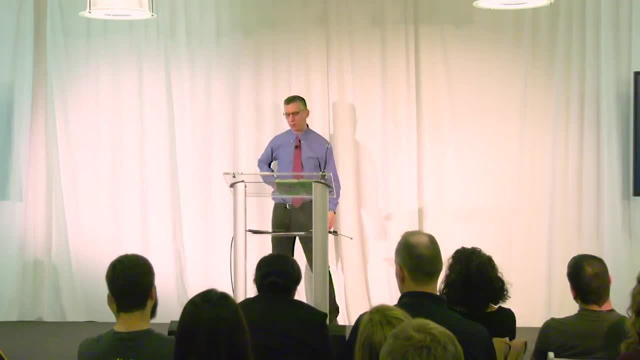 A lot of interesting stuff, like all our research, everything we do when we're not doing, all the other stuff that we're doing And when you- but here I'm framing it another way- I'm talking about how I want to help you, right.